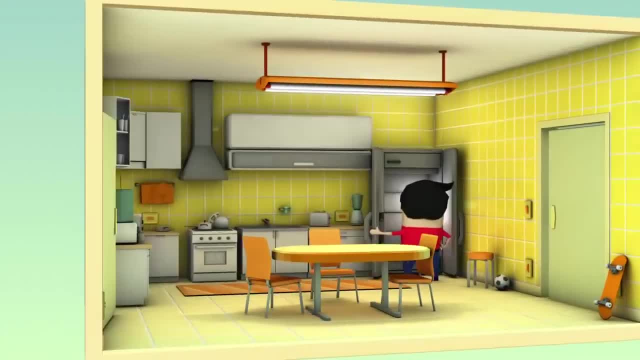 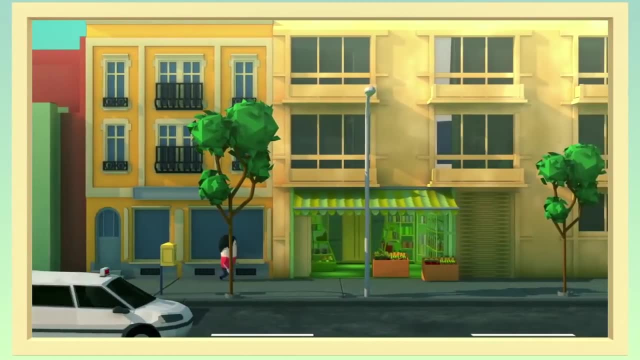 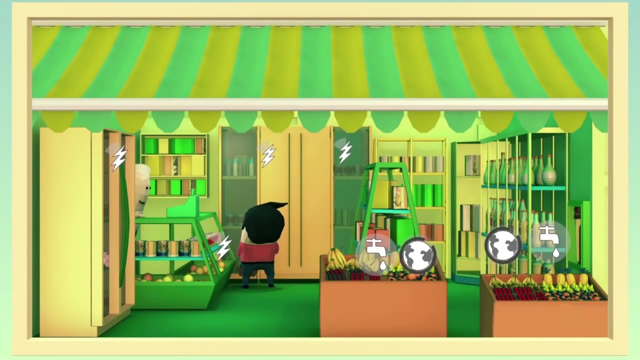 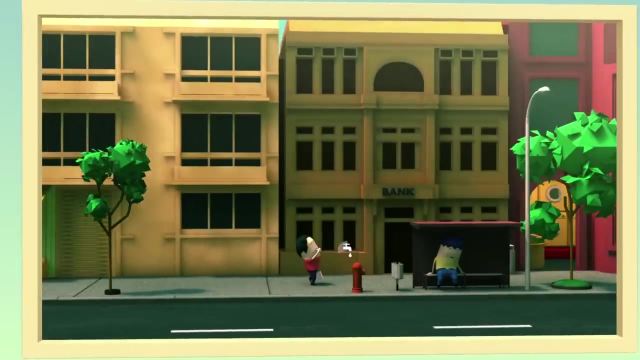 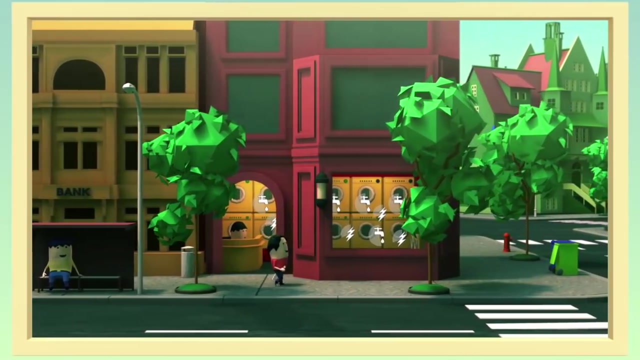 resources isn't exactly his strong point, But from the looks of it, food resources are also scarce here. It's time to think about resupplying, And it's difficult to choose from so many options. You may think that this yogurt container has a very short life between the supermarket. 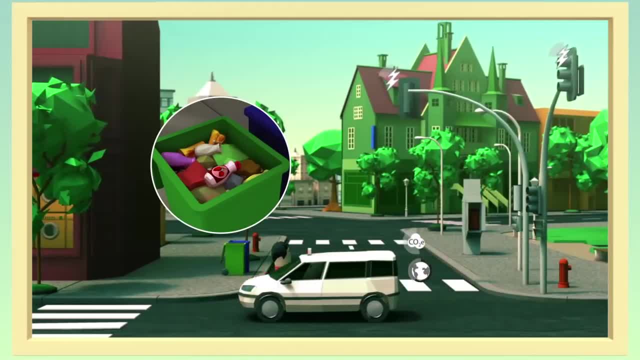 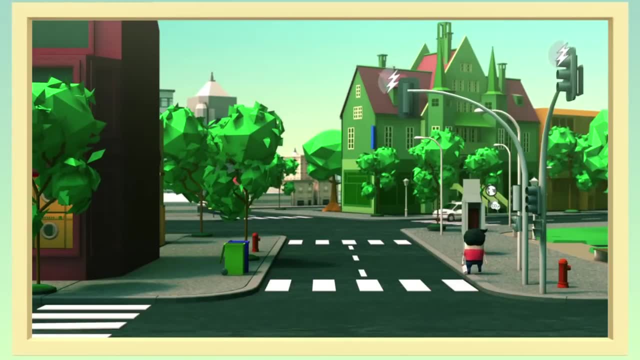 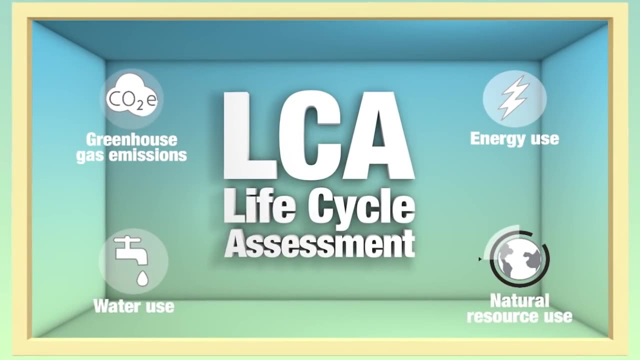 and the trash can. But who said that's how the story ends? And who said the supermarket was the start? There have already been many phases in this product's life cycle and many more are still to come. To better understand how this works and its impacts, a very efficient tool exists. 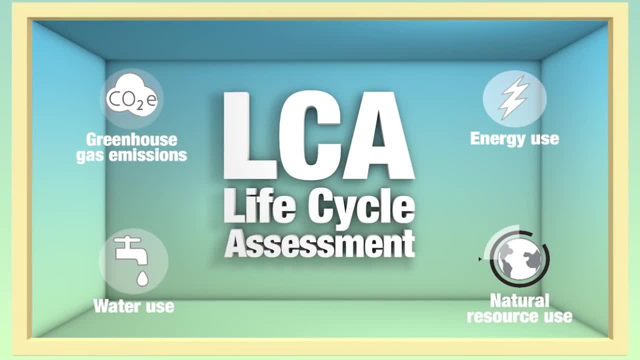 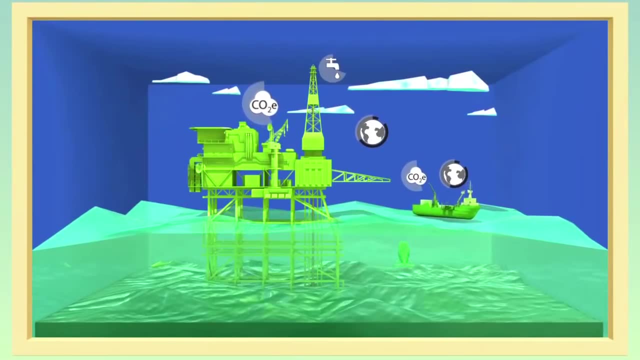 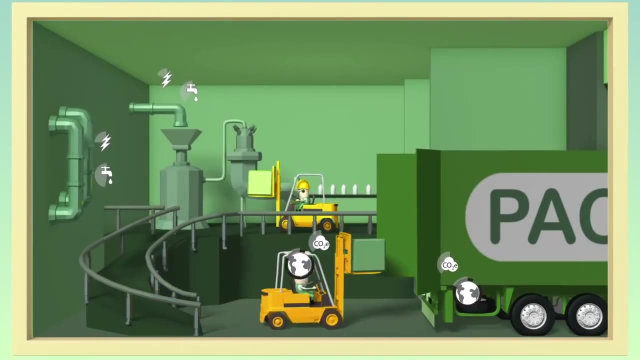 The Life Cycle Assessment. You want an example? Let's analyze the cycle of the very same yogurt pot. Everything starts with the extraction of the raw materials. Among other things, oil is used to make the plastic pot that will protect its contents. There's also the milk used to make the yogurt. 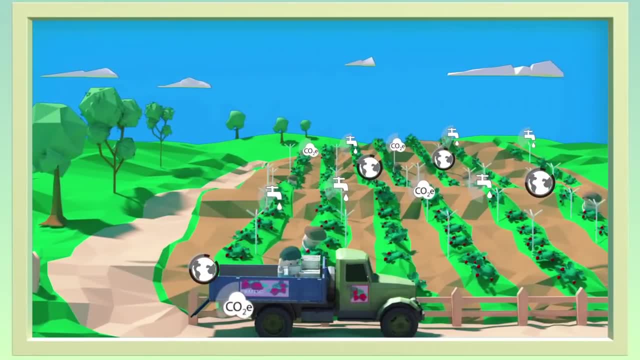 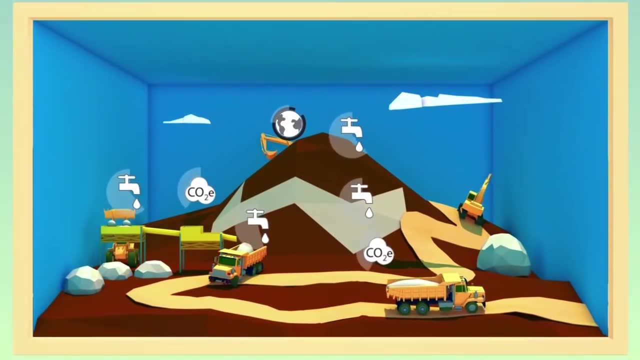 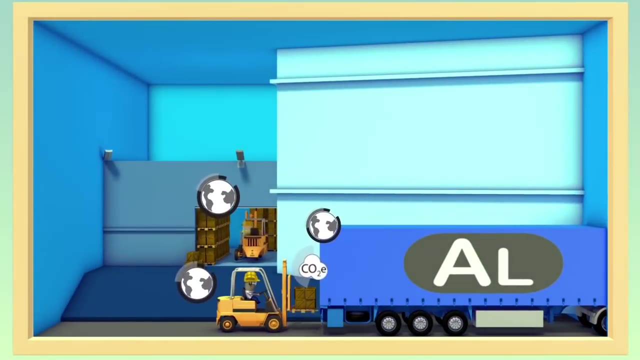 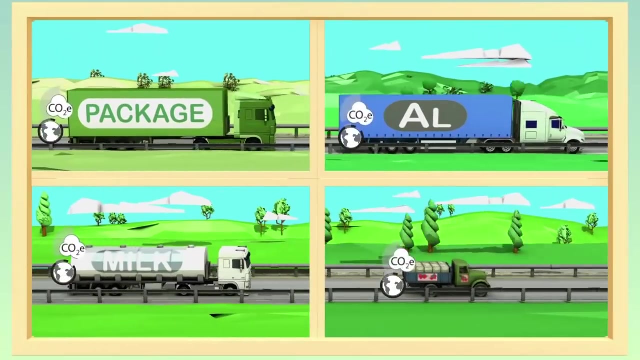 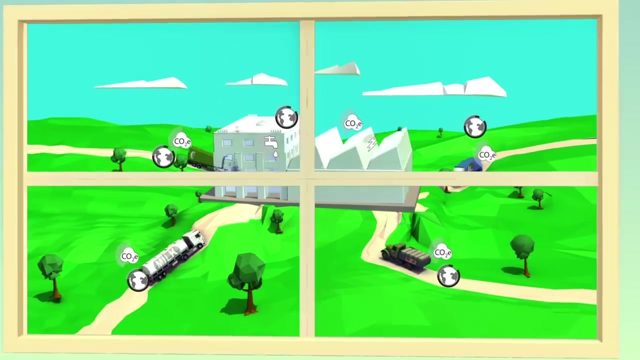 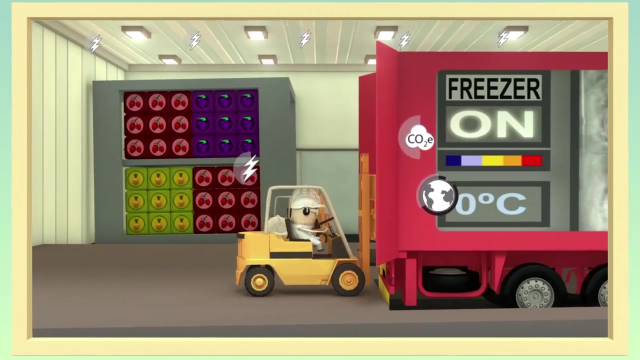 The strawberry for flavor, The aluminum foil lid to seal in the product. There's lots of different processes And each one has various kinds of impacts on the environment, And the cycle is only just beginning. At various moments there's need for transportation. 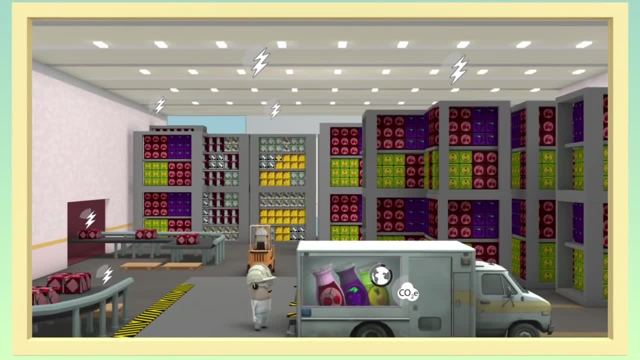 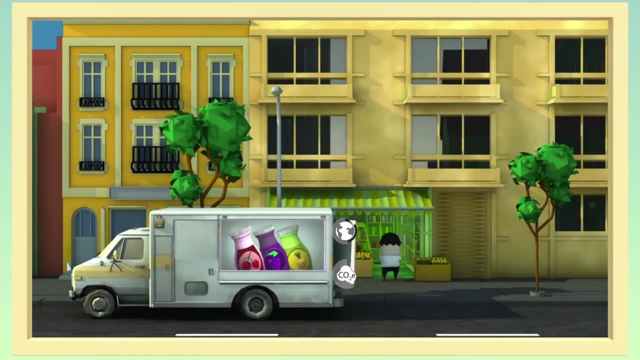 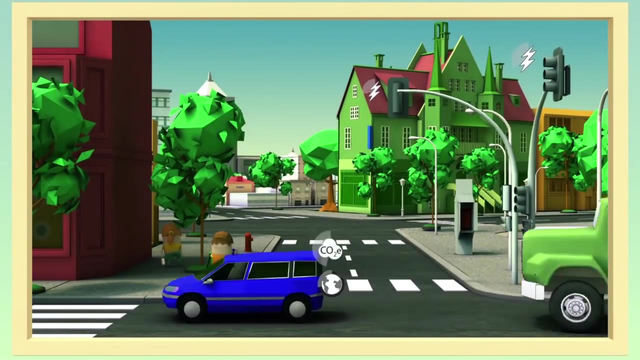 Then there's storage And distribution. It's a long way to reach the consumer And, like I said before, the story doesn't end with the trash can. The pot can be recycled and used to make a new product, With the cycle restarting or, more precisely, continuing.